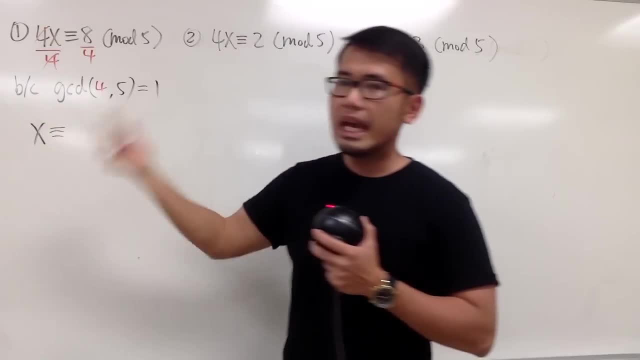 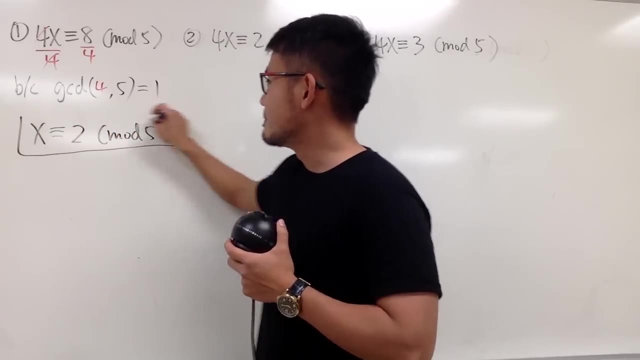 and you will have. x is congruent to 8 divided by 4.. It needs no introduction, which is just 2.. And of course you keep writing down the mod 5.. And this right, here is it, And usually we want to have this number. 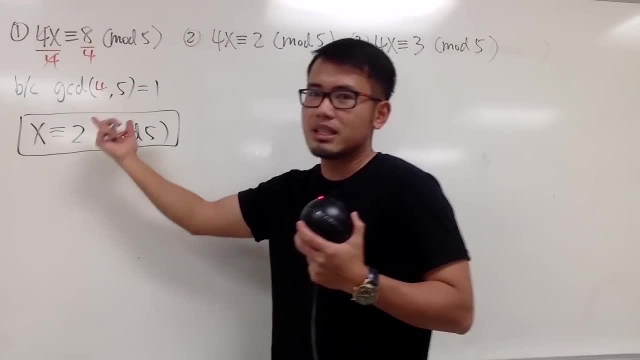 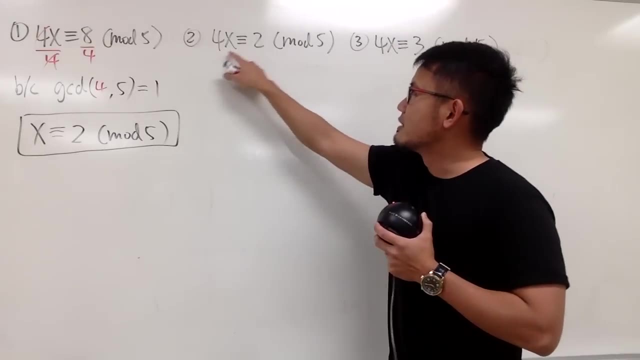 to be less than this number And, of course, keep it as positive as possible. But anyway, x is congruent to 2 mod 5, done. Next we have 4x is congruent to 2 mod 5.. 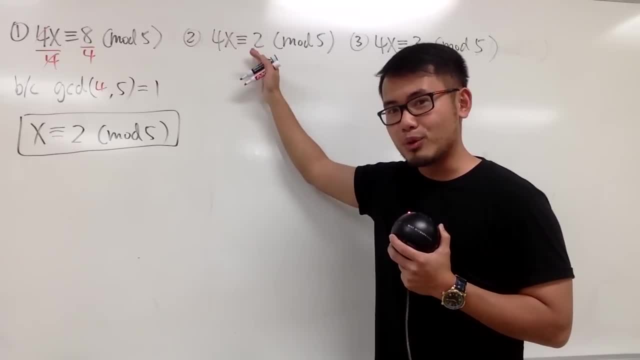 Well, in this case we have 4x is congruent to 2 mod 5.. In this case we cannot just divide by 4 on both sides, because 2 divided by 4 is 1 half. And remember, we are not doing fractions or decimals. 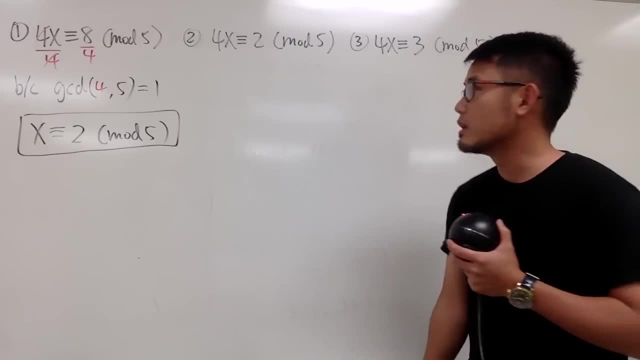 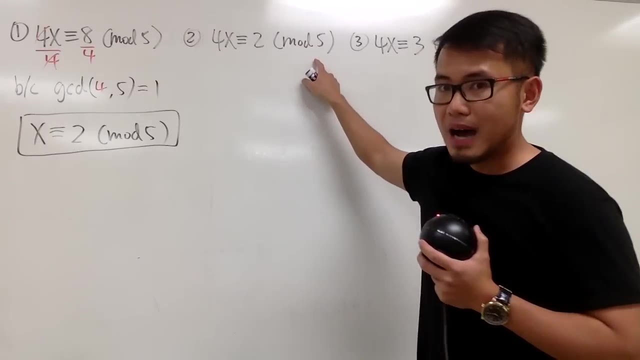 in the congruence world. So now we have to think about this carefully Here. hmm, it's 4x. The deal is, we can do 4 mod 5.. 4 mod 5, 4 is just pretty much smaller than 5, right by 1.. 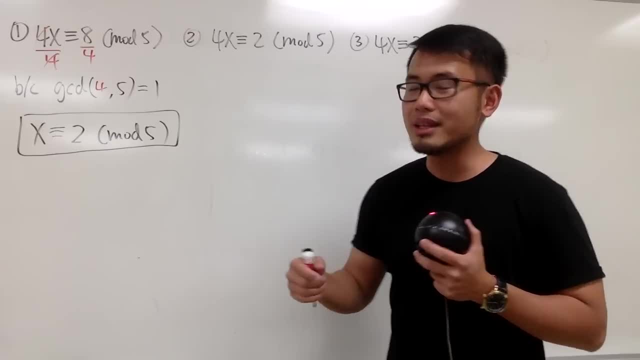 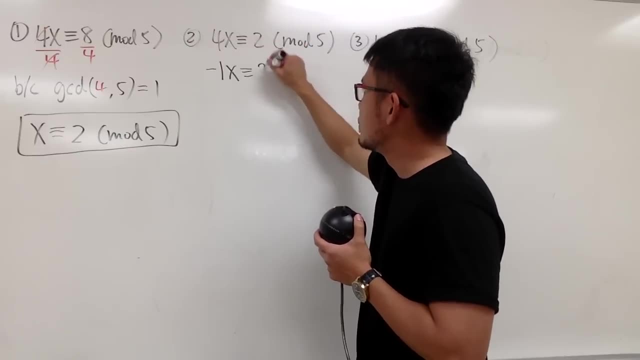 So you can just do 4 minus 5, which is negative 1.. So this right here is just going to be negative 1.. So this right here is just going to be negative 1x, And then you can maintain the mod 2,. 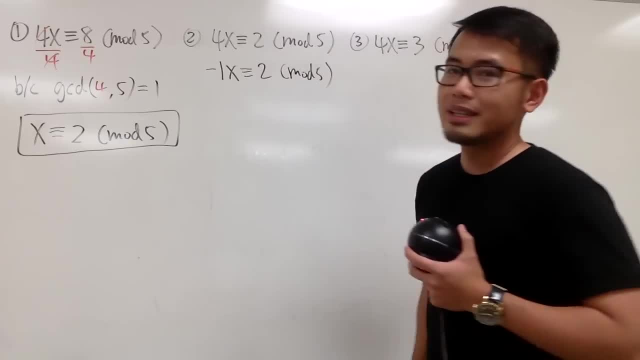 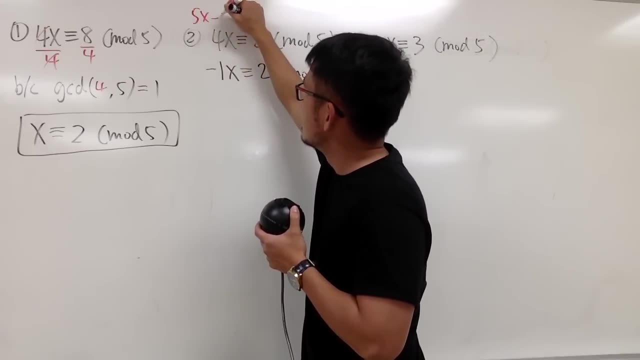 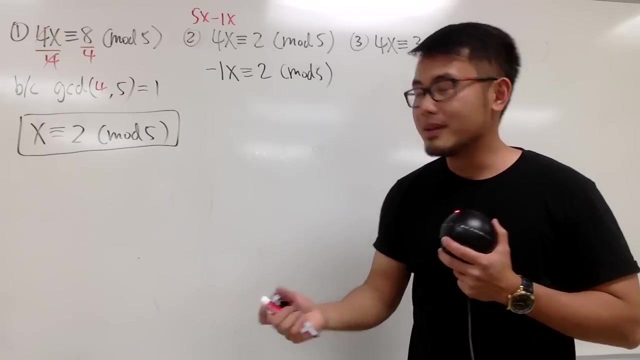 meaning the congruent to 2, and then mod 5.. This is legit because you can look at the 4x as 5x minus 1x, right, And you see, 5x, that's always going to be a multiple of 5.. 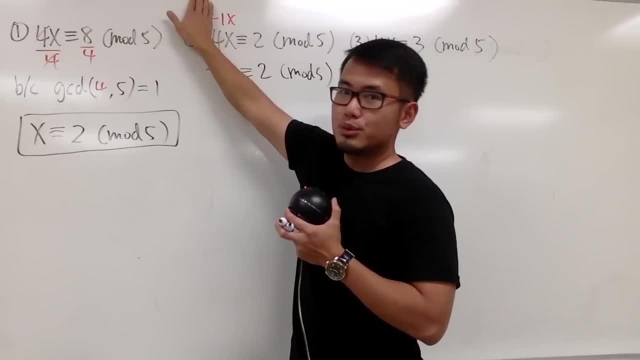 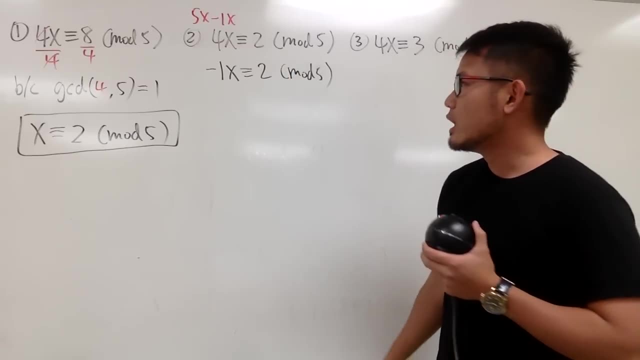 And in the mod 5 world- this right here, it's going to be 0. So you just get negative 1x And this is congruent to 2 mod 5, OK, And now we can divide both sides by negative 1.. 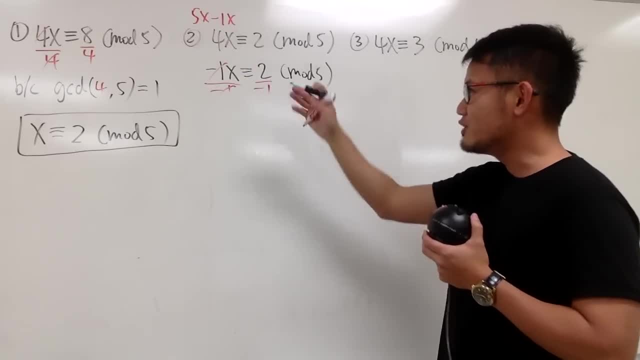 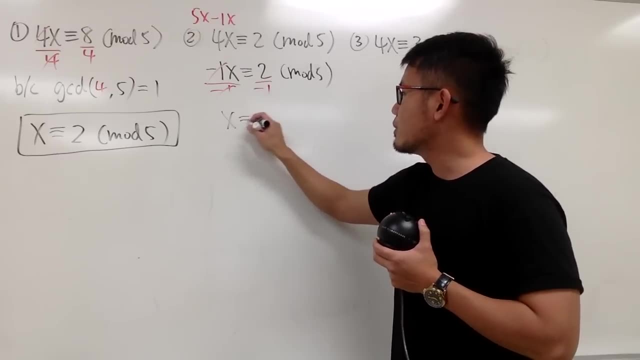 So this is also legit, right? So let's change the sign on both sides. it's OK. We can look at this as: multiply both sides by negative 1, same thing And you get. x is congruent to negative 2 mod 5.. 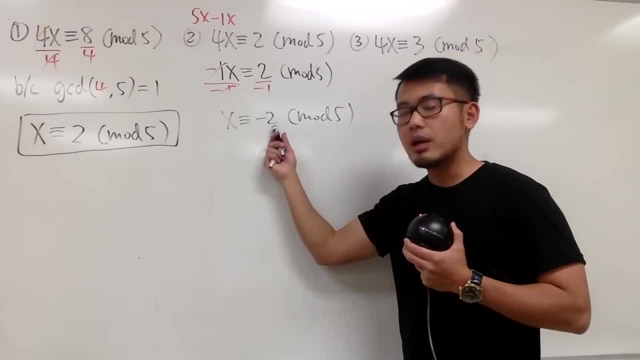 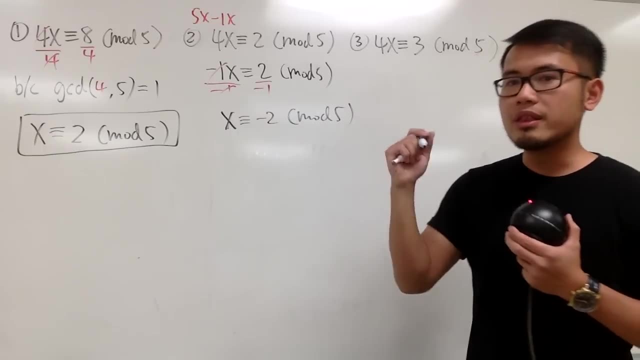 And, as I said, we want to keep this number as positive as possible. right, The x is by itself already, So you can look at this. So this is what we can do, Starting from negative 2, and just add 5 to it, which you get 3..